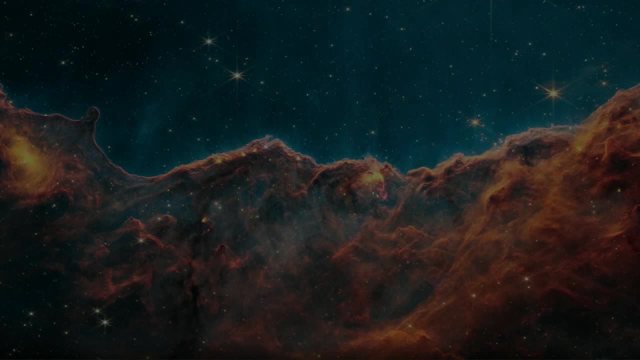 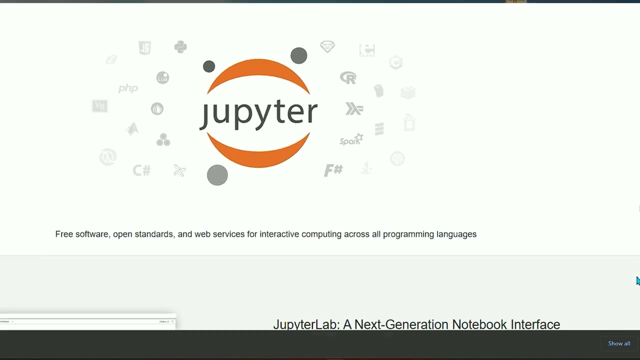 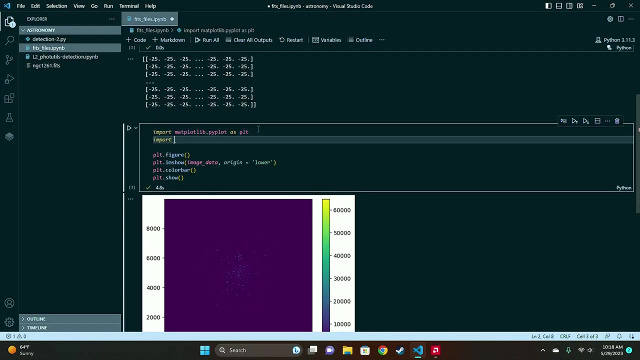 Hello everyone and welcome to this AstroPie tutorial. My name is Micah and in this video we will be going over handling and viewing FITS image files using Jupyter Notebooks. This is a first in a series of videos where we will learn how to use Python and AstroPie to handle raw space telescope data and perform aperture photometry. 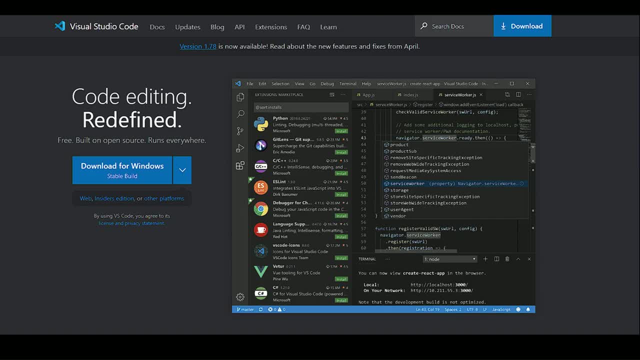 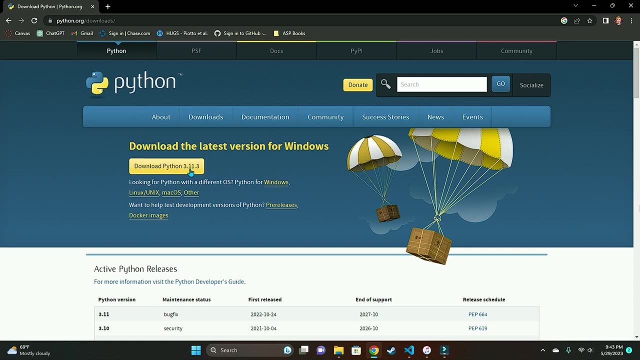 For this tutorial, you will need to install Visual Studio Code and Python. You'll need at least version 3.8 of Python, but I recommend installing the latest stable version At the time of this recording, that's Python 3.11.. 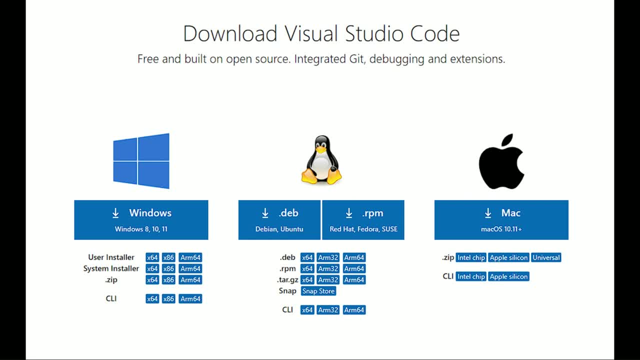 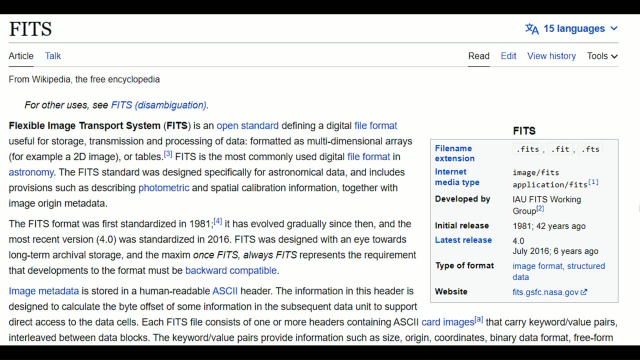 Now these programs are available for Windows, Linux and MacOS, and I'll include links to their download pages in the description. Finally, you will need to find a FITS file to work with. Once you get all that done, go ahead and open up Visual Studio Code on your computer. 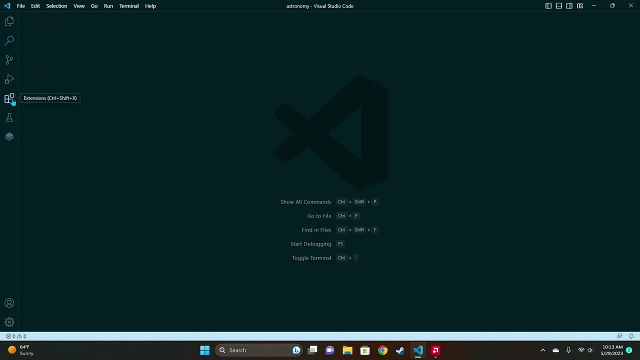 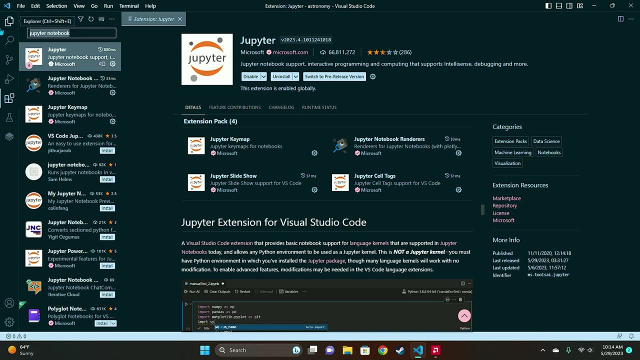 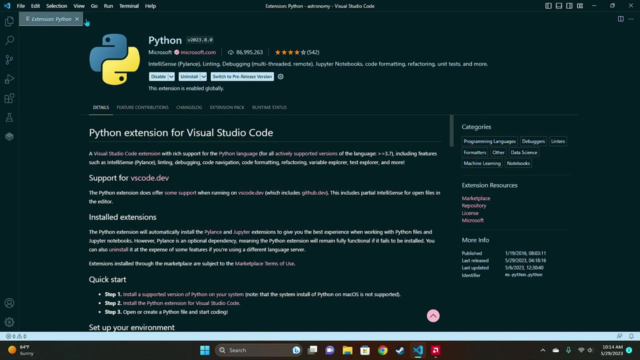 Then go over to the left here where it says Extensions. Click on that and you're going to want to install the Jupyter Notebook extension and the Python extension, This one right here. Once those are installed, you can go ahead and close that and then we're going to open up a terminal. 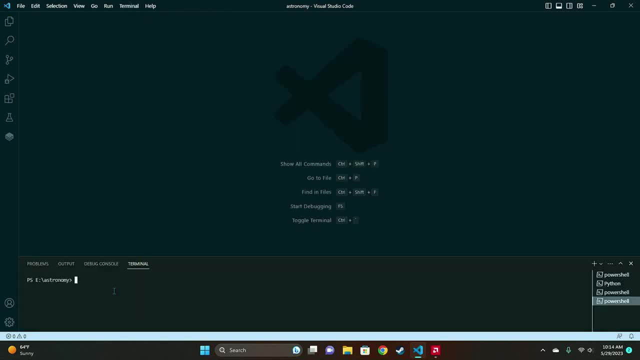 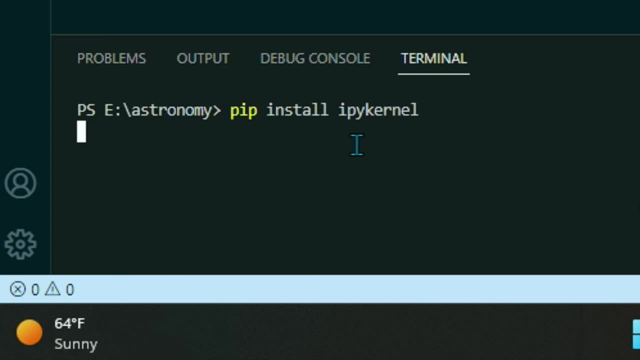 Click New Terminal there and you're going to type in a few codes. So the first thing you're going to do is pip, install ipy-kernel, and that will install the Python kernel for us, Which allows us to compile and run our code. 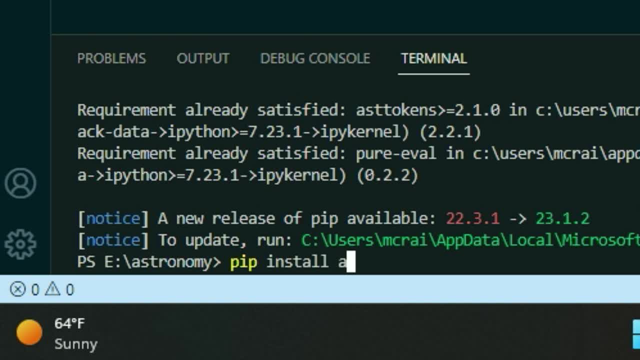 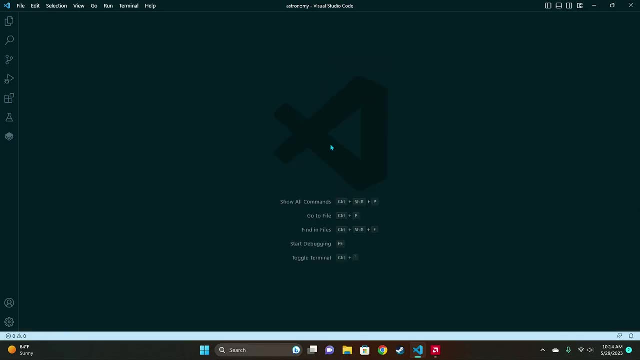 Then you're going to do pip install astropy And finally, pip install numpy. Okay, we now have all the packages that we need to start coding. So go over to your Explorer and you'll want to make sure that your current directory 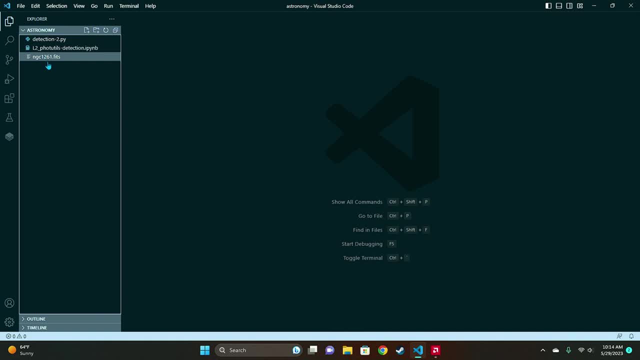 your working folder is open to where you have your fits image file, Which in my case is this file right here: ngc1261.fits. Then, once you do that, go ahead and click File and do New File and select Jupyter Notebook. 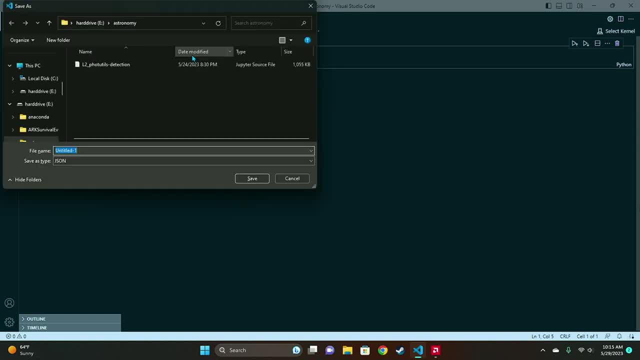 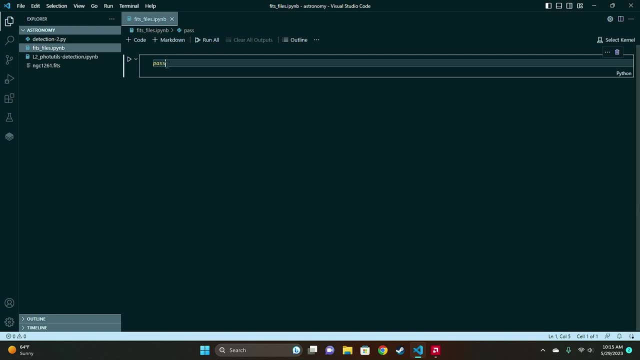 So the first thing I'm going to do is save this, and we'll just call it fits files. And now we have our Jupyter Notebook and we can begin coding. So the way Jupyter Notebook works is we have these different blocks of code. 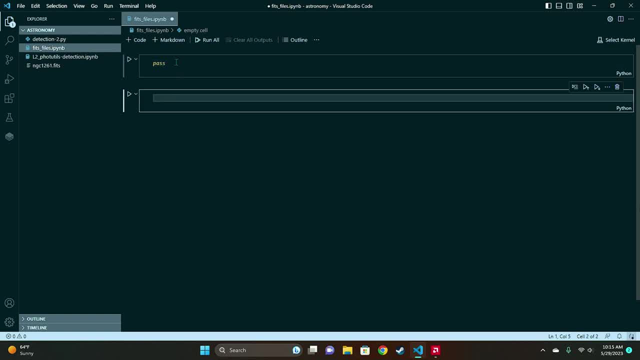 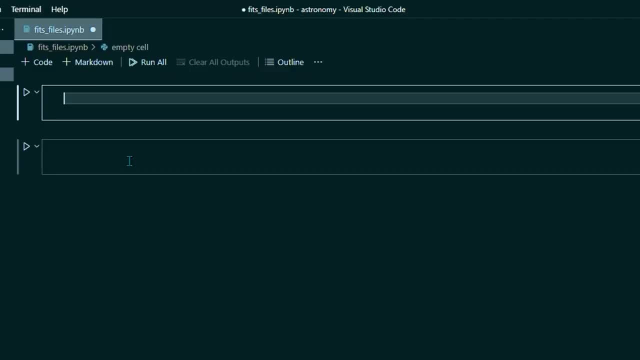 and we can just run these blocks individually. So it's just a really easy way to run and debug Python. So to begin coding, the first thing I'm going to do is import from astropyio- import fits, And this will give us our fits file tools. 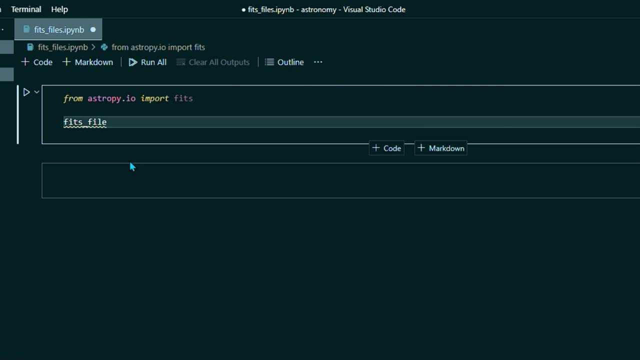 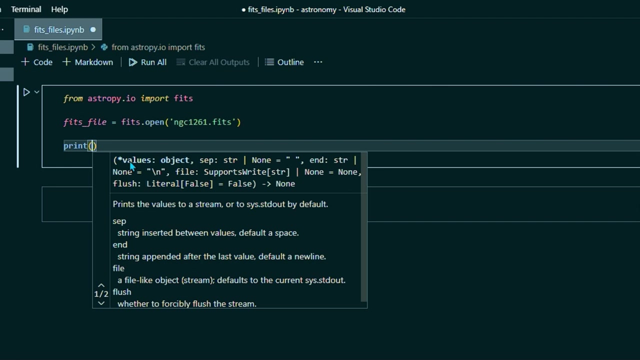 So then, to open our fits file, we'll do. fits file equals fitsopen, and then the name of our fits file: ngc1261.fits. And now let's go ahead and print that to see what it looks like. All right? 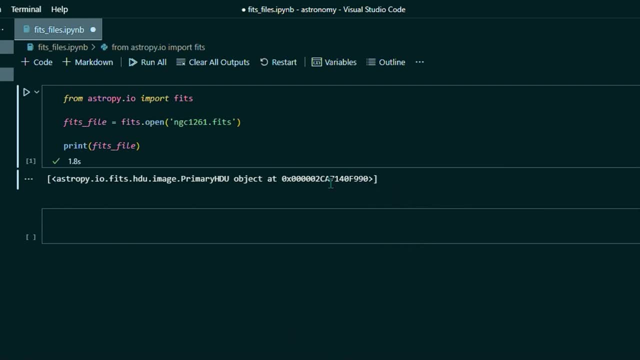 So we have this list here with a single item in it, and that's not very useful. So what we can do now is go up here and change this So our fits file. sorry, we'll go into our next block of code. 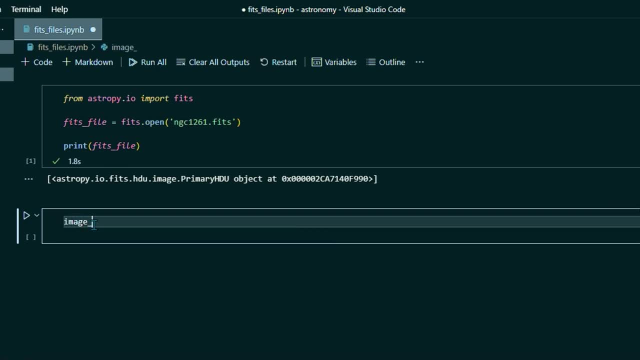 And now we want to get our image data. So we'll make a variable called image data Set that equal to fits file 0.data, And it adds that random underscore right there. We don't want that. I don't know why it does that, but just make sure you delete that, or else your code won't work. 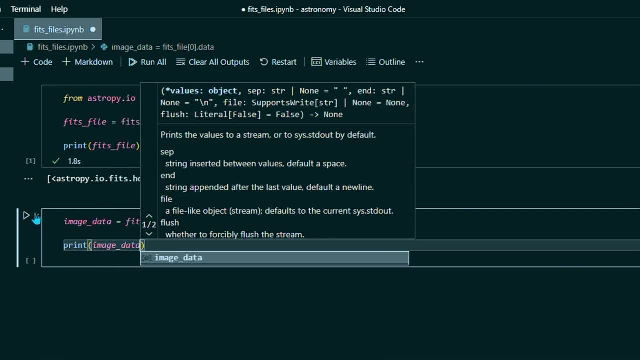 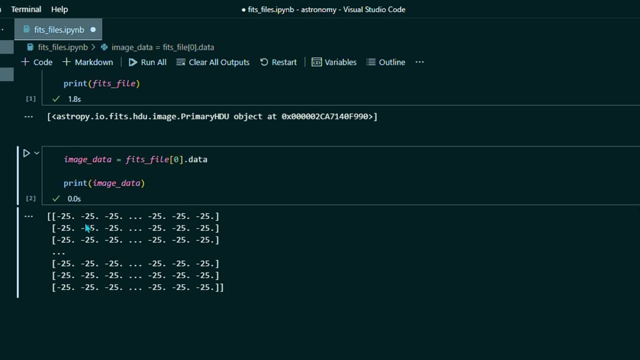 Now let's print that, Okay. So now we have a rather long list with a bunch of numbers And basically what this is. it's every pixel in our fits image and it's assigned a value of brightness. So now that we have our data, 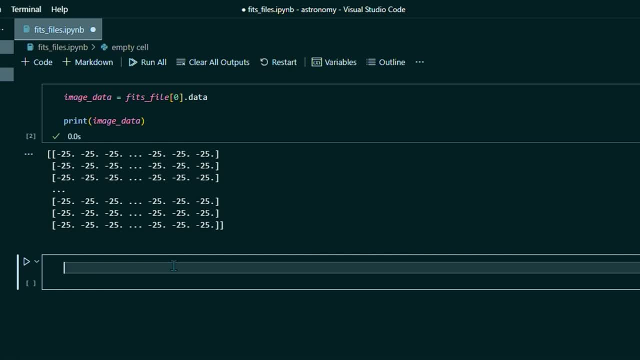 what we can do is use matplotlib to view that as an actual image. So let's do: import matplotlibpyplot as plt And then what we'll do is type pltfigure- Don't forget those open- close parentheses- pltimshow- And then we'll do image data. 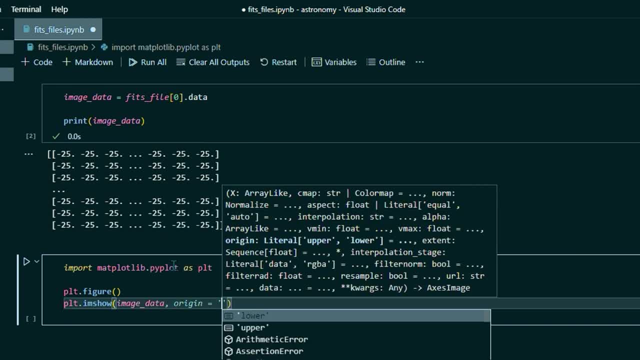 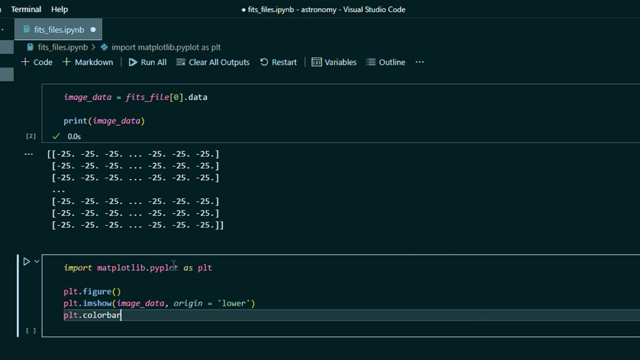 origin equals And then quotes lower, And then we'll also want to plot a color bar And then you'll type pltshow And also we'll need those open- close parentheses after color bar. So this one will take a little while to run. 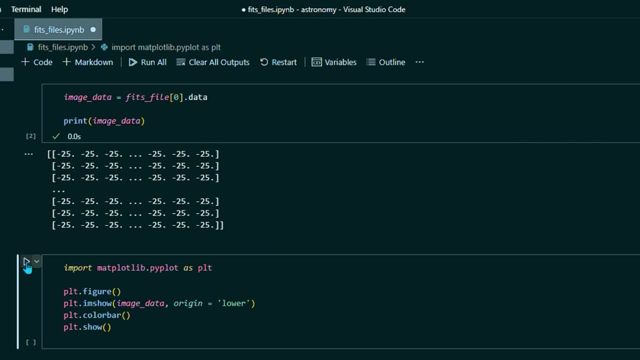 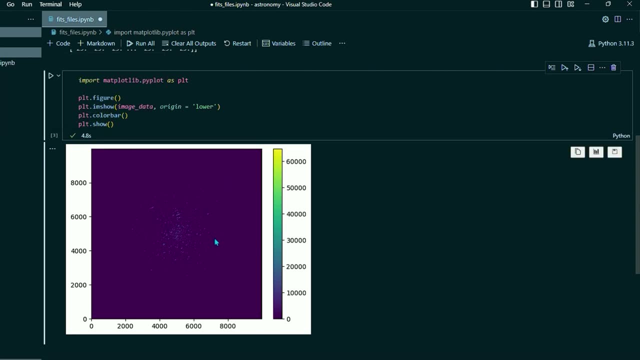 On my computer it'll take about 30 seconds, So I'll just skip ahead till that finishes running. But don't be concerned if this takes a while to run. Okay, So I lied, It took about 4.8 seconds. 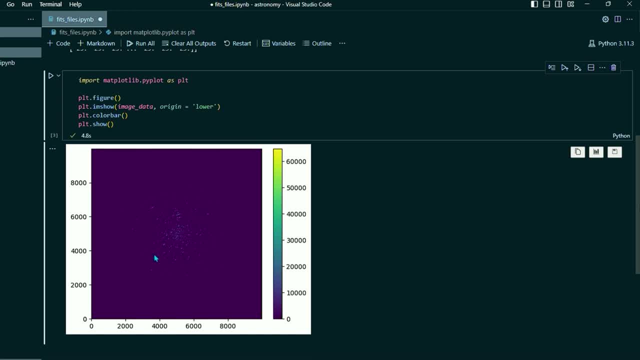 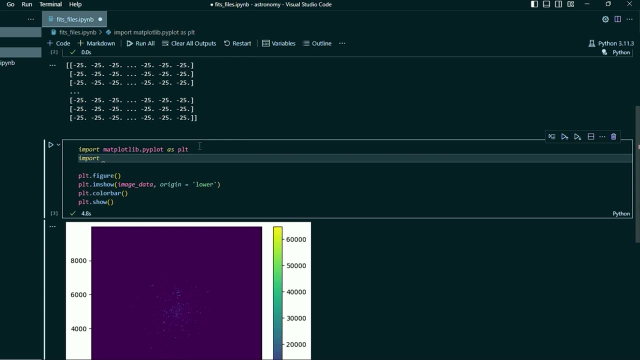 But here we have this image right here And it doesn't look like much. It's kind of hard to tell what's going on here. So we're going to do a few things to fix that. So the first thing we can do is we'll go up here and we'll import. 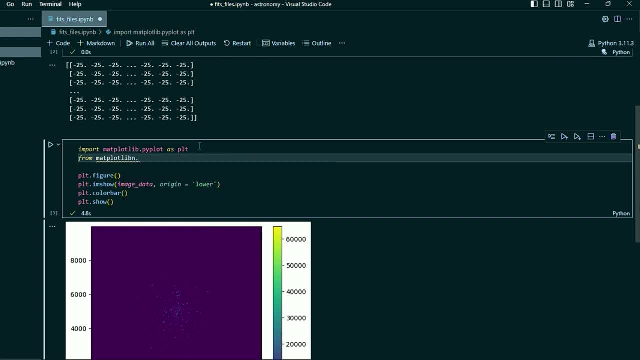 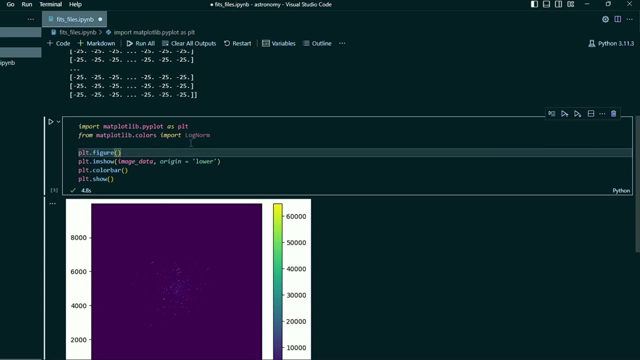 from matplotlibcolorsimportlogpy- import log norm, And this will allow us to display our image with a logarithmic fit which basically just allows us to see the dimmer stars. So you import log norm And then right in here in our plotmshow command. 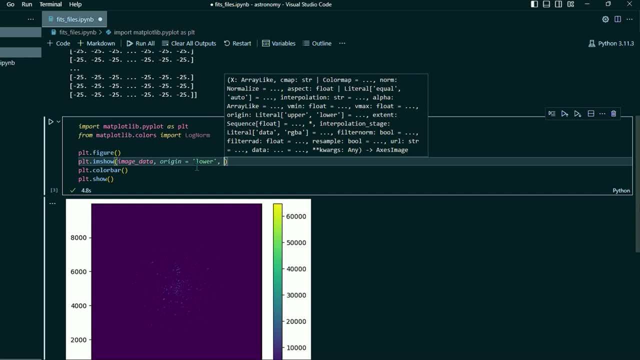 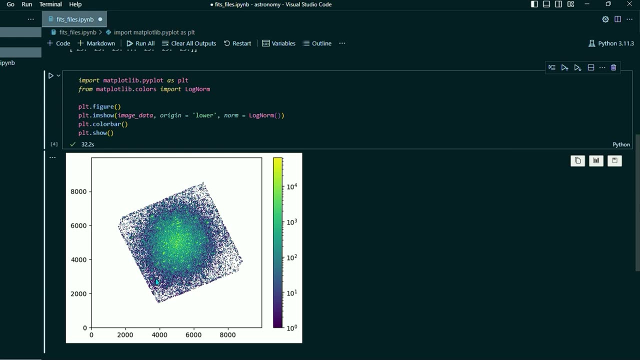 we'll add a comma And then another item. We'll do: norm equals log, norm open, close parentheses. So if we run this again, Okay, That time it did take over 30 seconds, But we can see here that we can see a lot more going on. 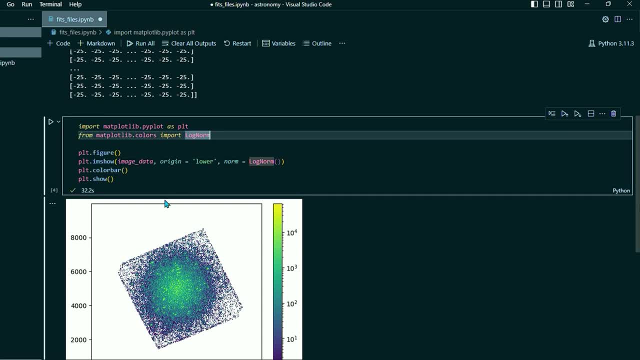 Now there are some funky colors going here, So another thing we can do just to make it a little easier to look at, is we can do. Let me add another comment here. CMAP equals grays. Make sure you spell gray with an E. 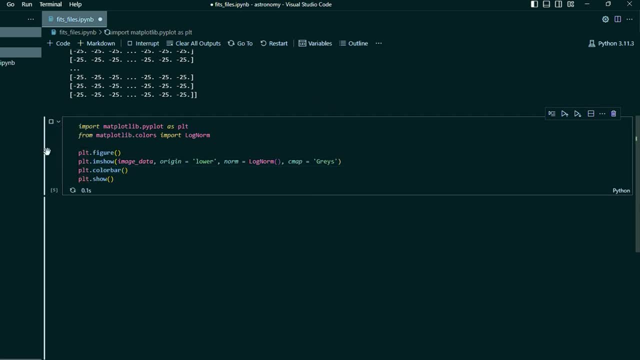 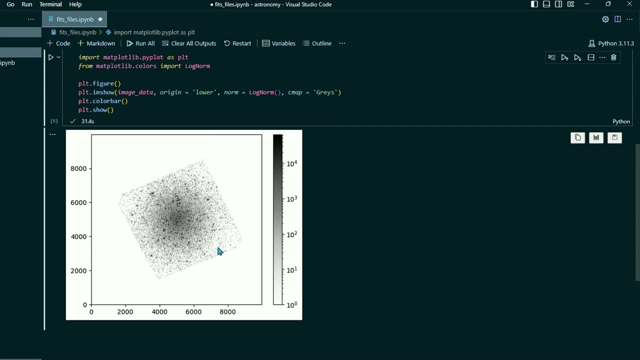 And if we run this again- And I'll fast forward until it finishes, All right. And now we see that everything is in black and white And that makes it a little bit easier to see what's going on. We can see clearly where there are stars and where there's not. 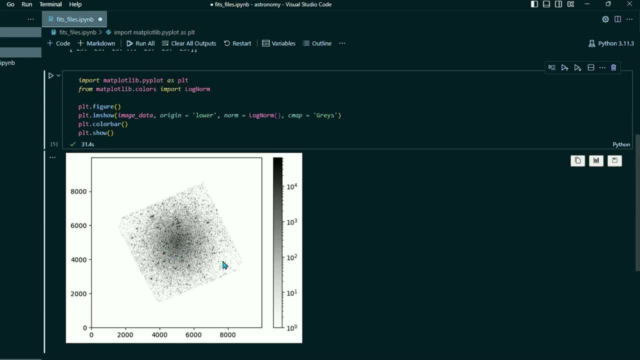 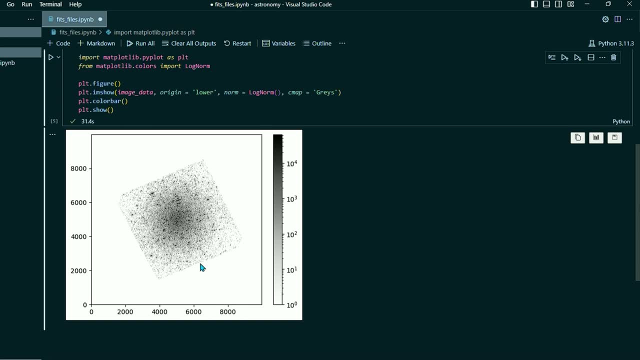 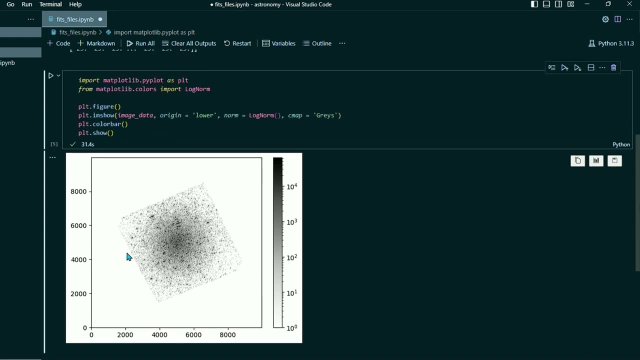 And we can see where there's more densely packed stars. So this is still, though, a lot to take in at once. It is still very small, And so we can't really see super well what's going on, So the next thing we're going to do is we're just going to define a smaller section of this. 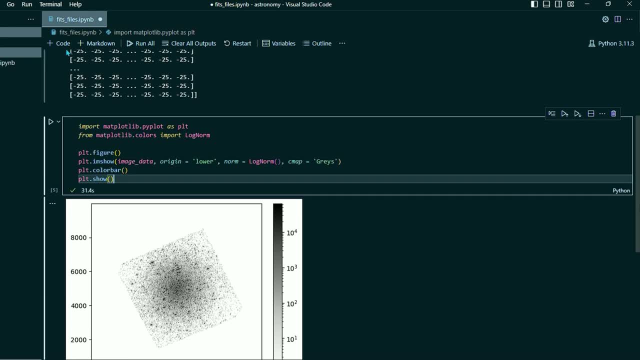 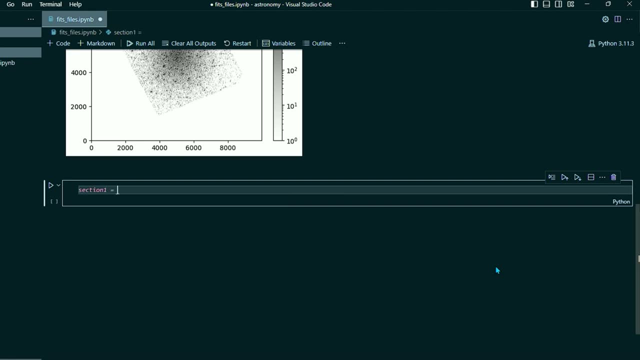 so that we don't have to deal with the whole thing at once. So I'm going to go ahead and create another block And we're going to create a variable called section one, And section one is going to equal image data, And then we're going to define X and Y coordinates of this data.